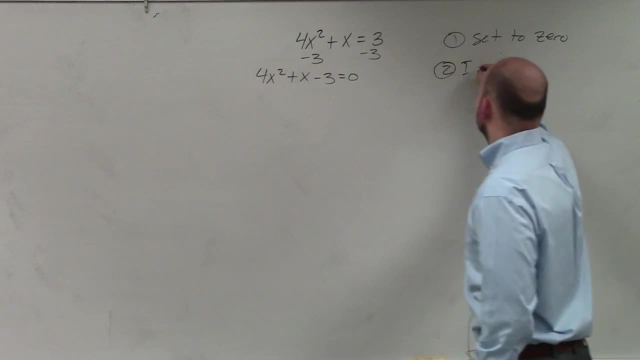 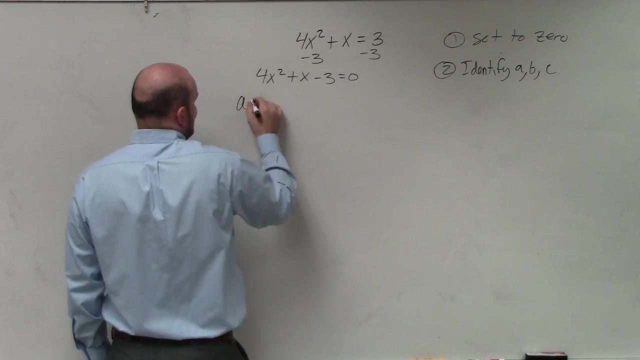 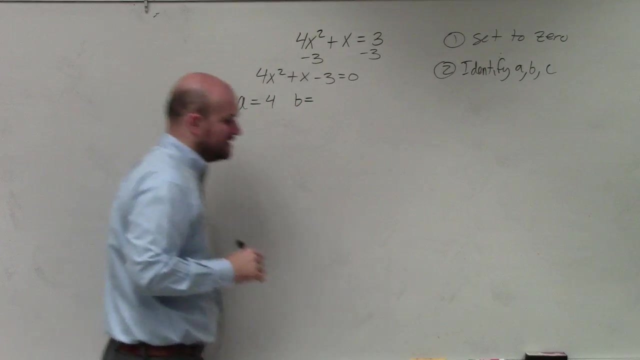 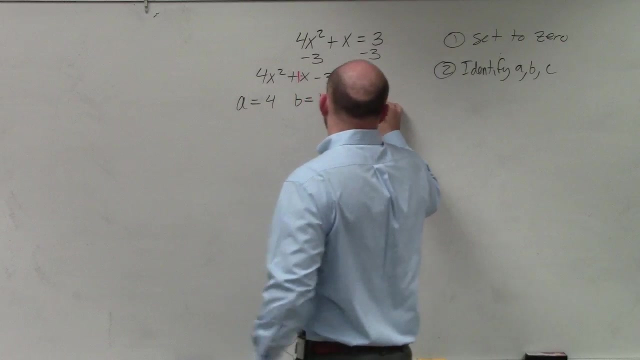 three equals zero. Step number two: identify A, B and C. So in this case, A, remember, is the coefficient of my quadratic term, which is four, B is the coefficient of my linear term, which is one, and C is equal to negative three, which is my constant. Step number three: 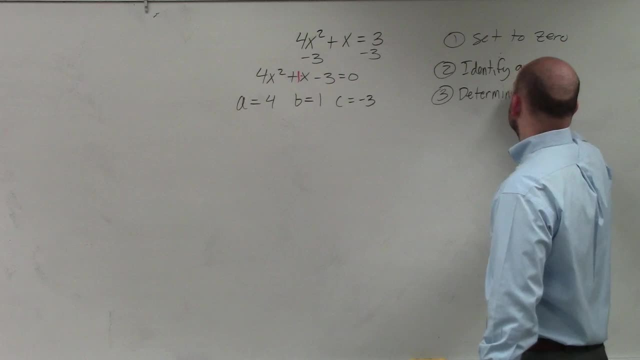 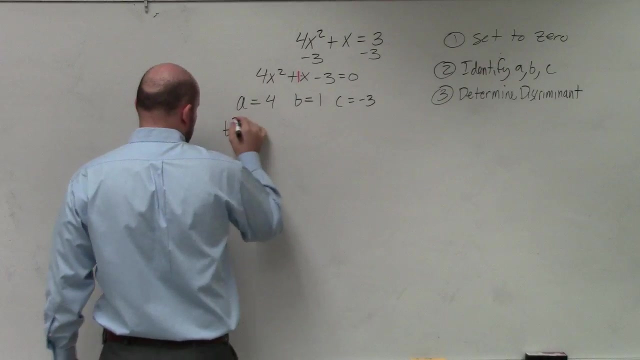 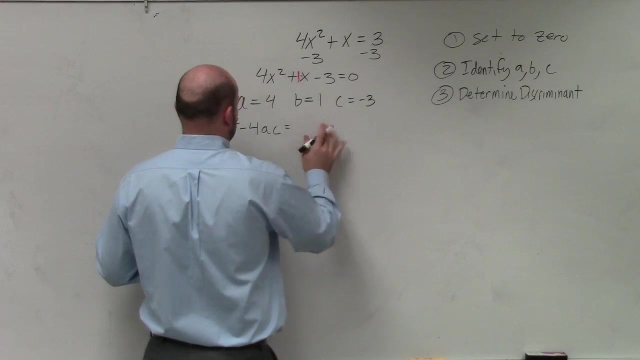 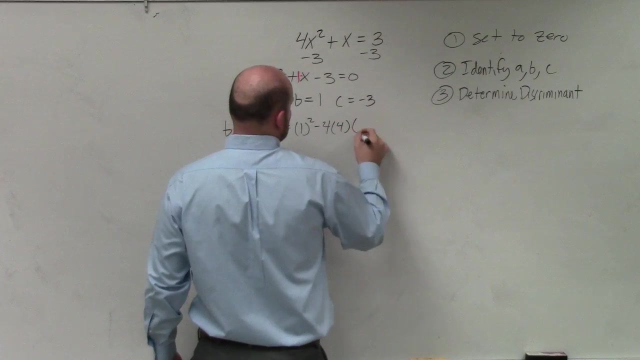 determine discriminant. So you guys remember the discriminant: That's just B squared minus four times A times C. So in this case that's going to be one squared minus four times A times C. Ooh, cucaracha Got it. 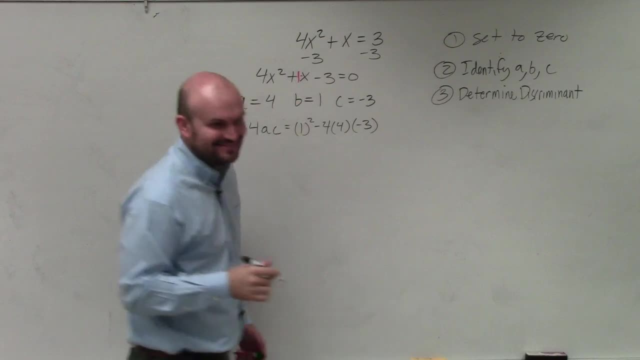 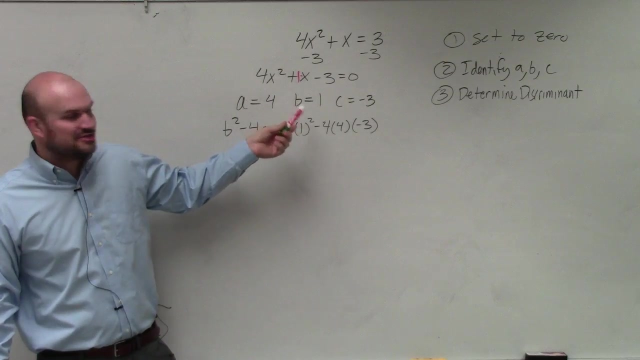 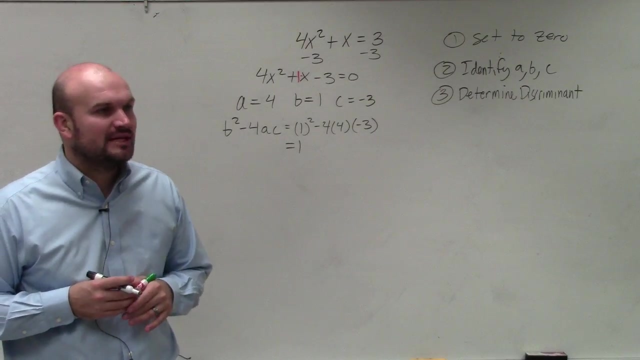 That's a cucaracha, Okay, Alright. so, guys, guys, let's try to finish up. I have five minutes left. Julian, Julian, Julian, Julian, Julian. Okay, So one squared is one, Let's do this. 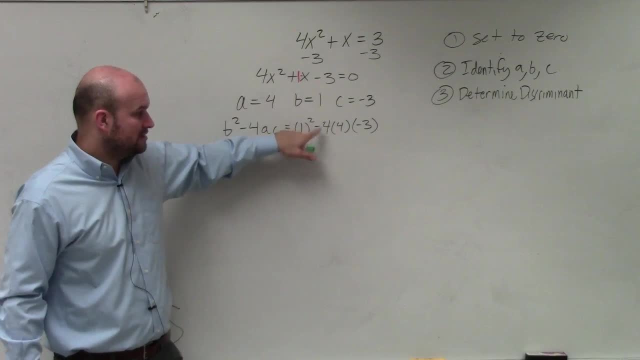 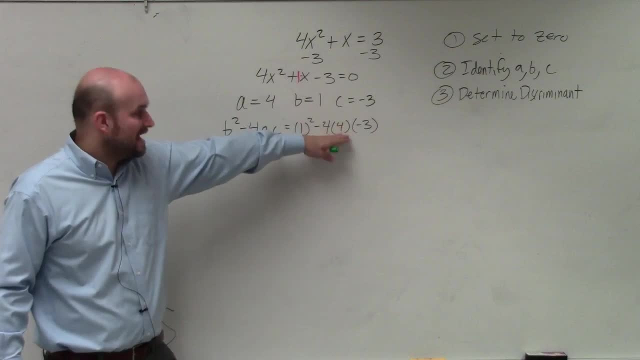 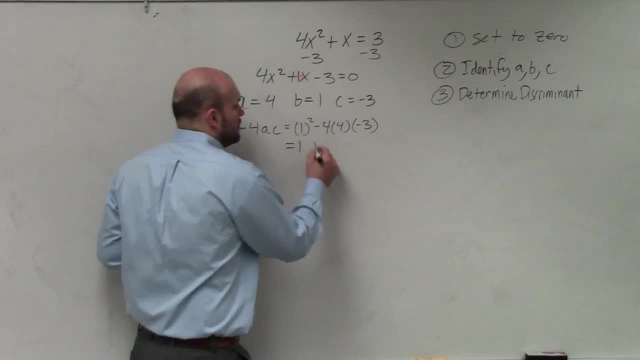 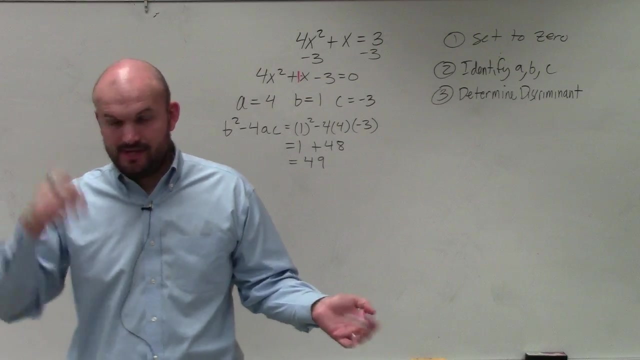 negative. three is going to be positive: 48.. One plus 48 is 49.. 49.. Is 49 a square number, McKenzie? Yes, Thank you, Look over here. Yes, 49 is a square number, So I'm not asking unless. 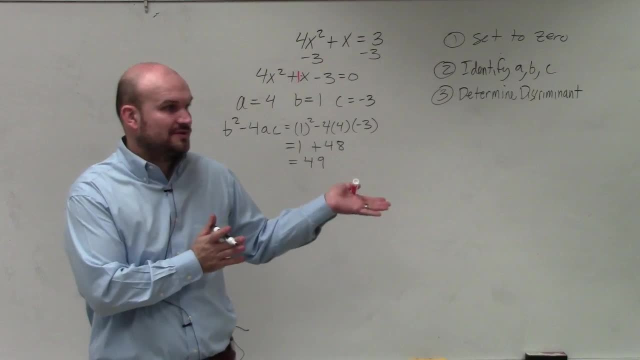 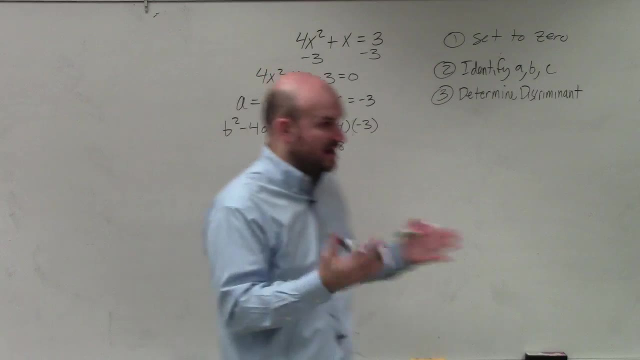 I tell you to write down what type of solutions are. you don't have to, But you guys should. hey, there's going to be two real rational solutions. Okay, good, So now what we need to do is we actually want to find the solutions. 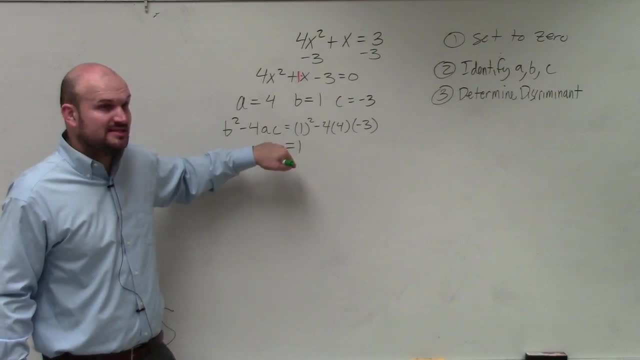 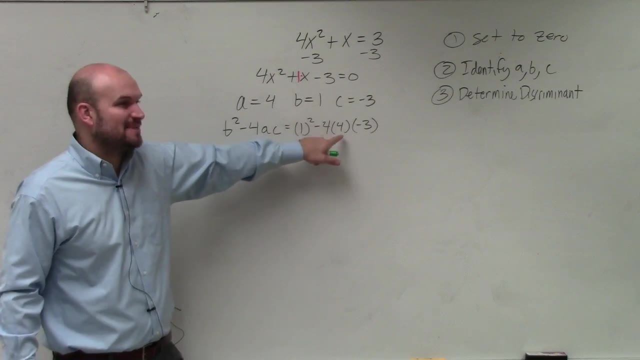 Okay, So one squared is one. Let's do this step by step, because here's where students make mistakes. Negative four times negative four, I'm sorry, negative four times positive four is Negative 16.. Negative 16 times negative three is going to be. 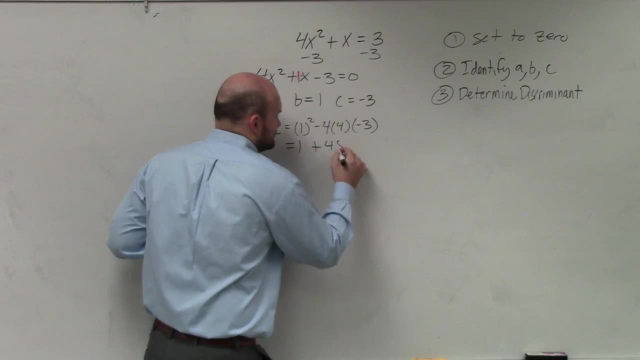 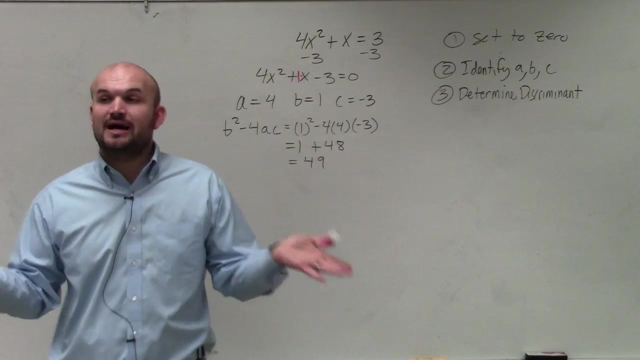 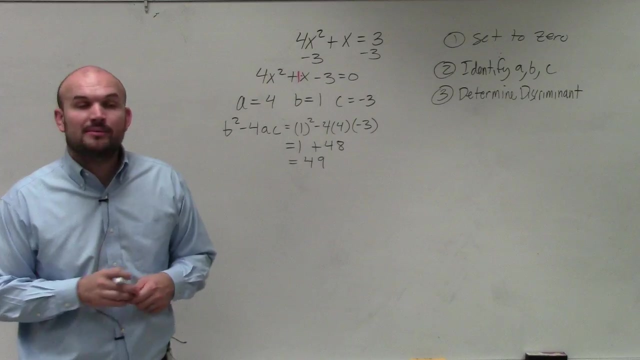 Positive: Positive: 48.. One plus 48 is 49.. Is 49 a square number, Mackenzie? Yes, Thank you, Look over here. Yes, 49 is a square number, So I'm not asking unless I tell you to write down what type of solutions are. you don't have to. 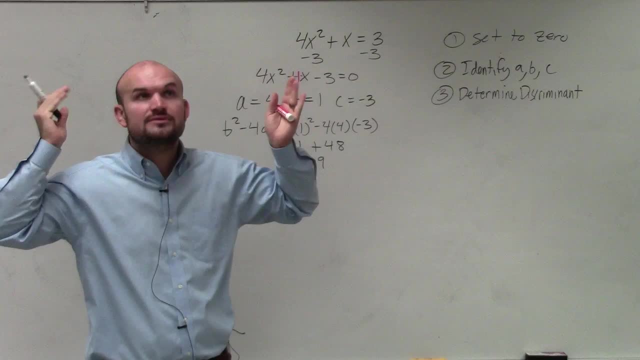 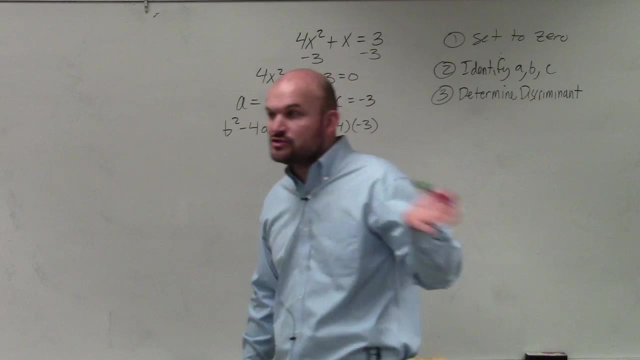 But you guys should know: hey, there's going to be two real rational solutions, Okay, good. So now what we need to do is we actually want to find the solutions, Rather than just saying, hey, There's two real rational solutions, we're actually going to find the solutions. 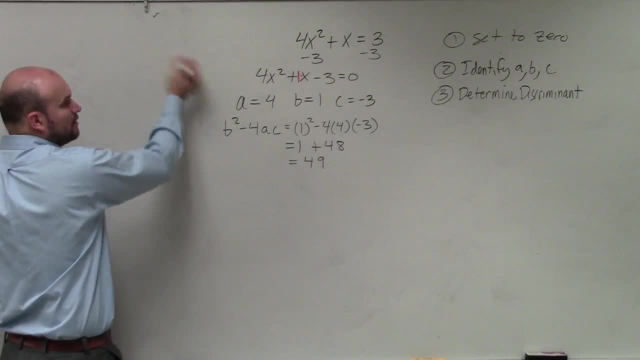 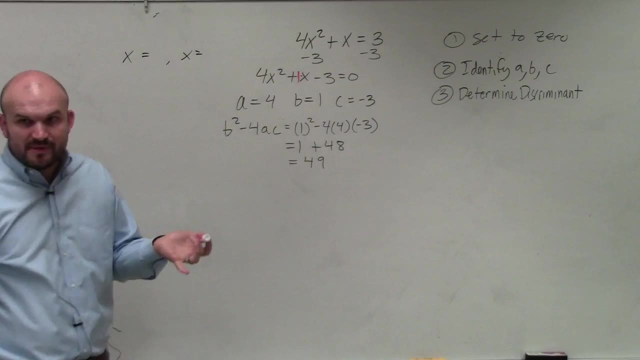 Now remember, guys, when you were solving a quadratic. remember at the end of the quadratic you always said: x equal this and x equal that. right, You guys remember that Solving a quadratic always at x equals. So what we're going to do is we're going to use the quadratic formula is actually another method. 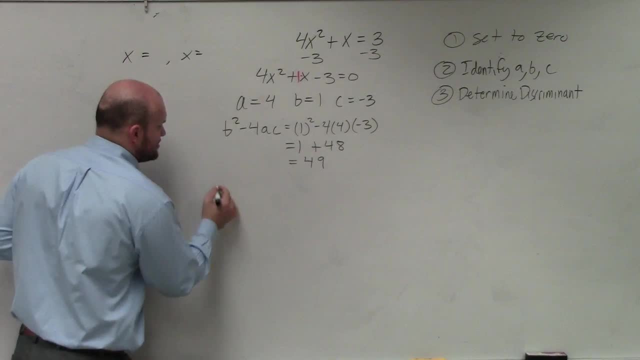 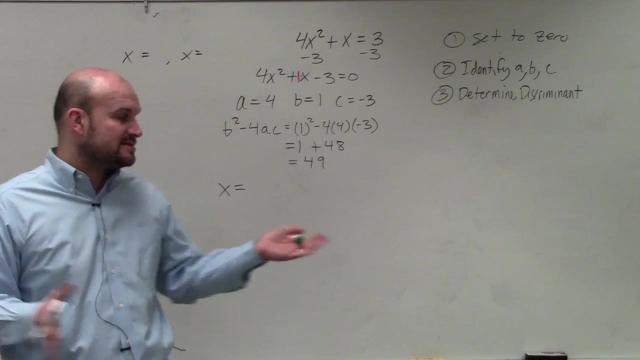 that we're going to be able to use to find all of them. But I want you guys to understand that the quadratic formula is going to tell you the solutions for x- So it's going to be x equals- And then to find all the solutions, and we'll talk more about this next class. 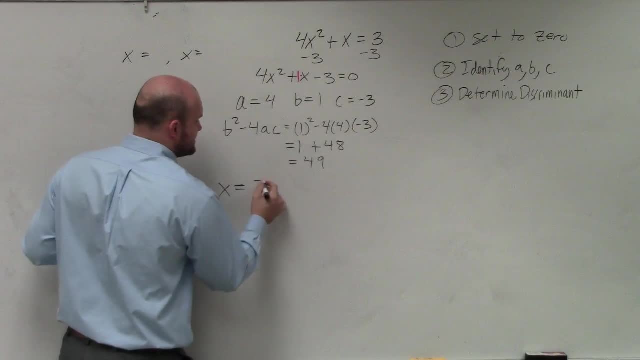 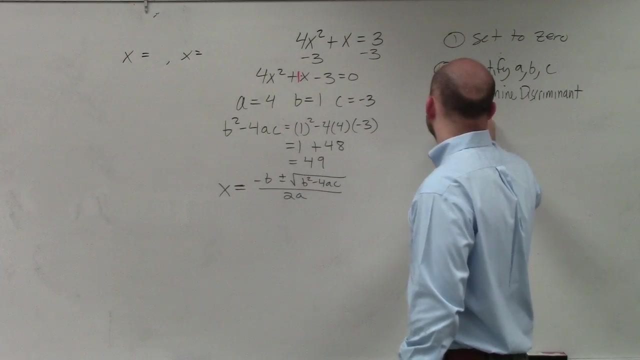 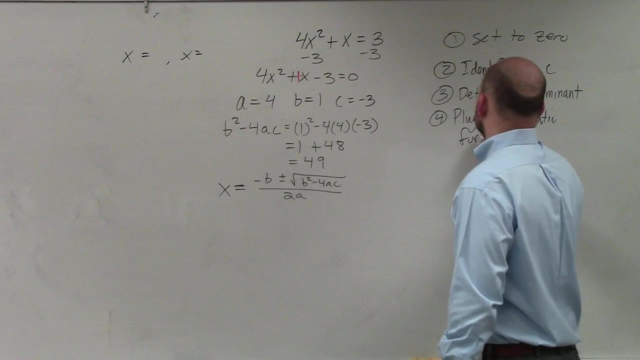 we're going to find all the solutions. You're basically, the quadratic formula is opposite of b, plus or minus, the square root of b, squared minus 4 times a times c, all over 2 times a. Okay, So What I want you guys to understand. 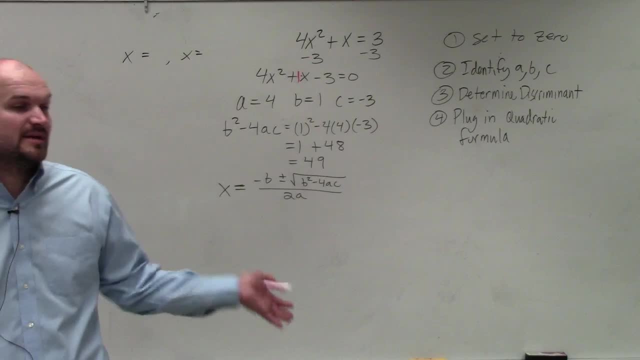 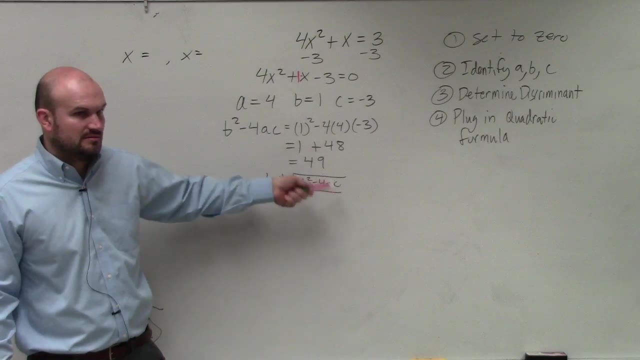 when you guys write down the quadratic formula which you are going to have to know on a test, It is not going to be given to you. Do you guys see that the number under the square root is actually the discriminant? Do you guys see that? 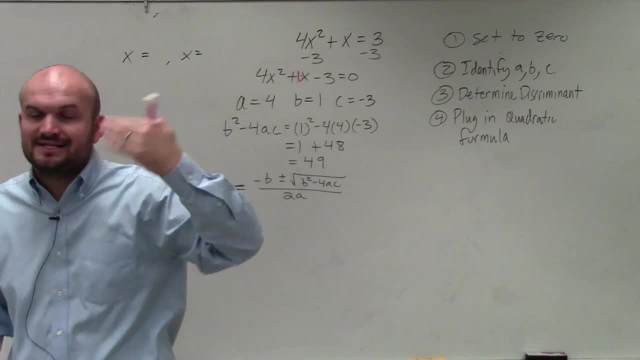 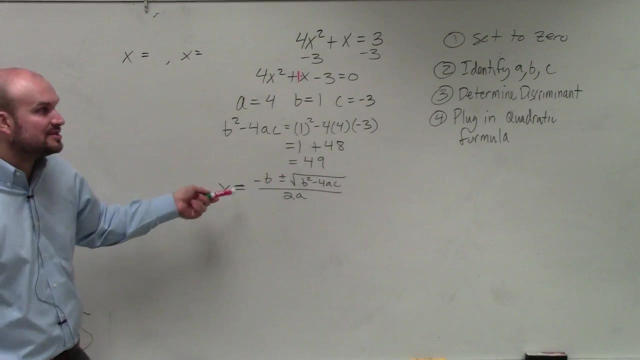 So guess what? By doing the discriminant, not only did that help us identify the type of quadratic or the solutions, but that also did half of our work for doing the quadratic formula to find the solutions. Now I just plug in my remaining values. 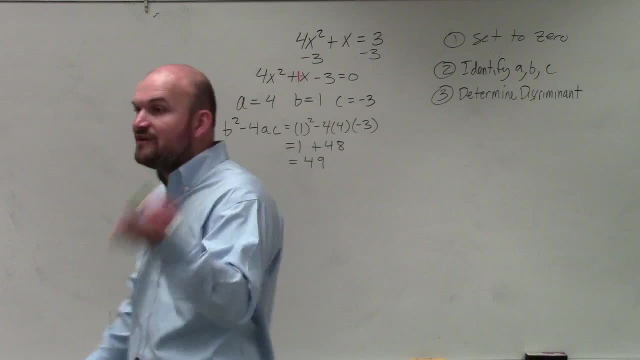 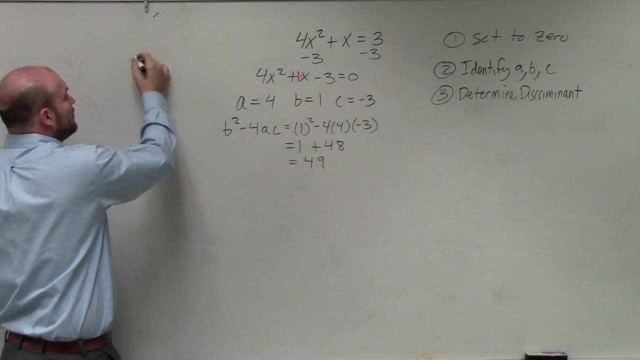 Rather than just saying, hey, there's two real rational solutions, we're actually going to find the solutions Now. remember, guys, when you were solving a quadratic. remember at the end of the quadratic you always said: x equal this and x equal that right. 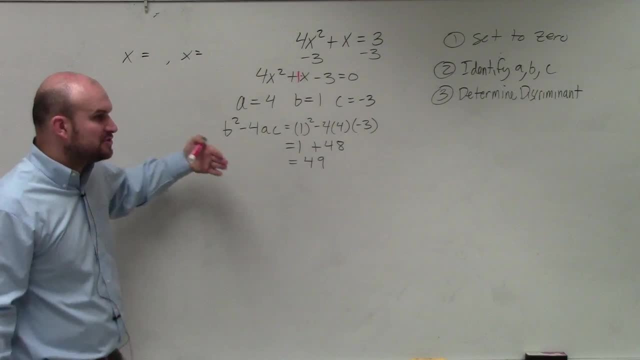 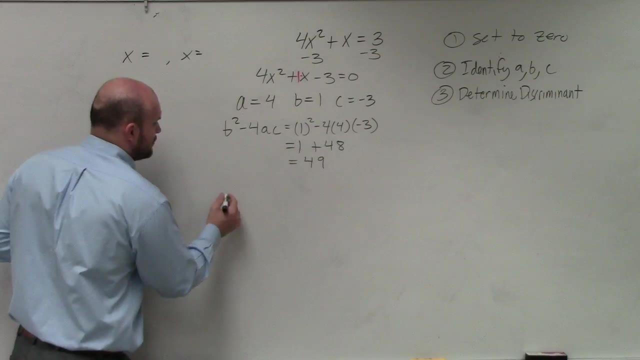 You guys remember that Solving a quadratic always at x equals. So what we're going to do is we're going to use the quadratic formula is actually another method that we're going to be able to use to find all of them. But I want you guys to understand that the quadratic formula 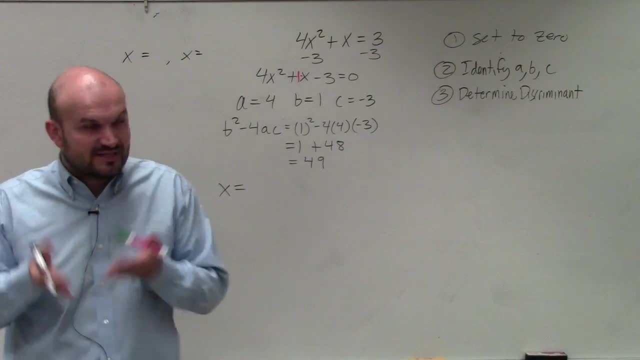 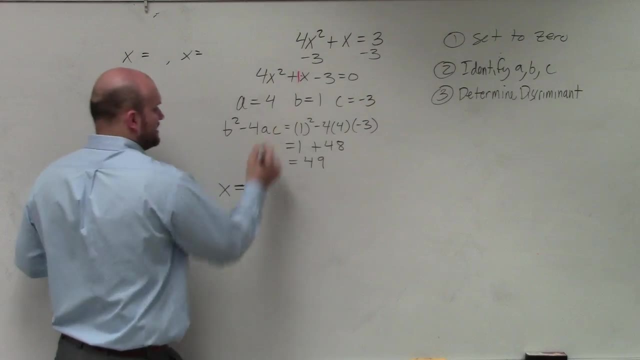 is going to tell you the solutions for x, So it's going to be x equals, and then to find all the solutions, and we'll talk more about this next class, but to find all the solutions you're basically: the quadratic formula is opposite of b, plus or minus the square root of b, squared. 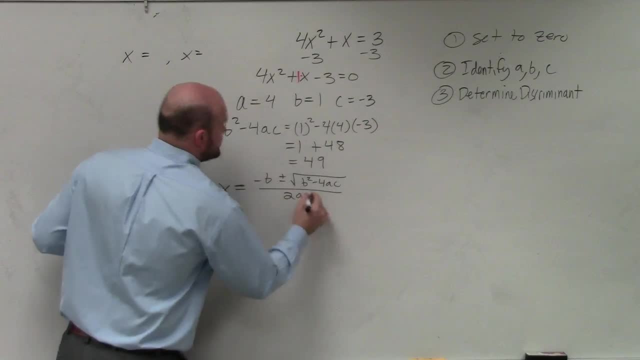 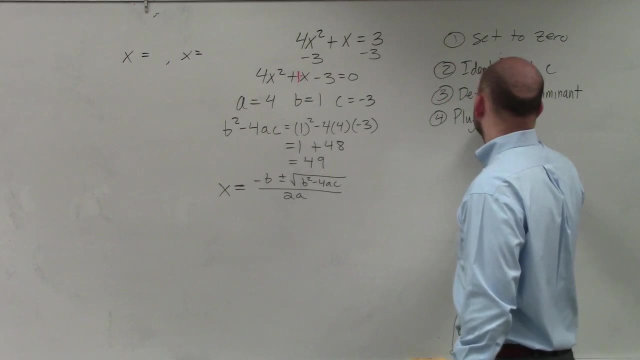 minus 4 times a times c, all over 2 times a. So what I want you guys to understand when you guys write down the quadratic formula which you are going to have to know on a test, It's not going to be given to you. 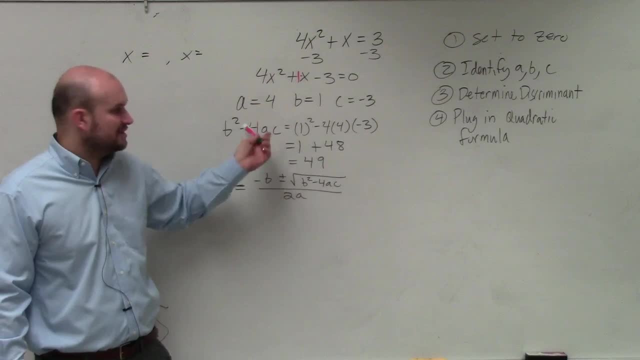 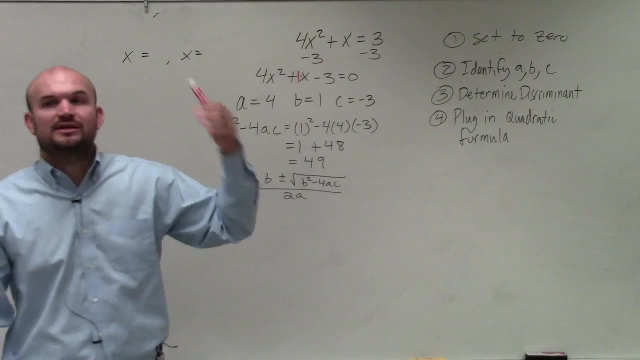 Do you guys see that the number under the square root is actually the discriminant? Do you guys see that? So guess what? By doing the discriminant, not only did that help us identify the type of quadratic or the square root, but it also helped us find the solution for x. 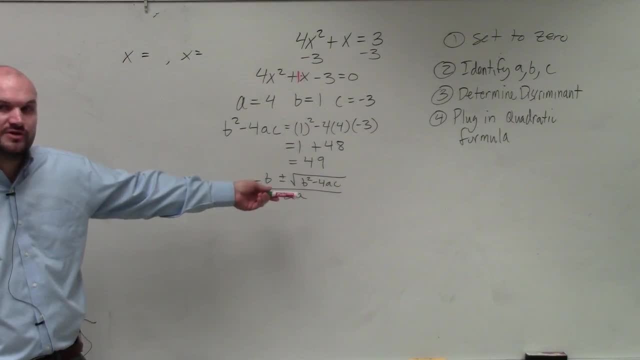 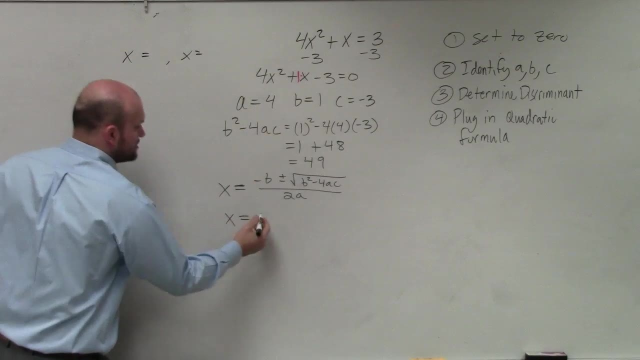 So that's what we're going to do. We're going to do the solutions, but that also did half of our work for doing the quadratic formula. to find the solutions. Now I just plug in my remaining values: Opposite of b: b is 1, so that's going to be negative, 1, plus or minus. 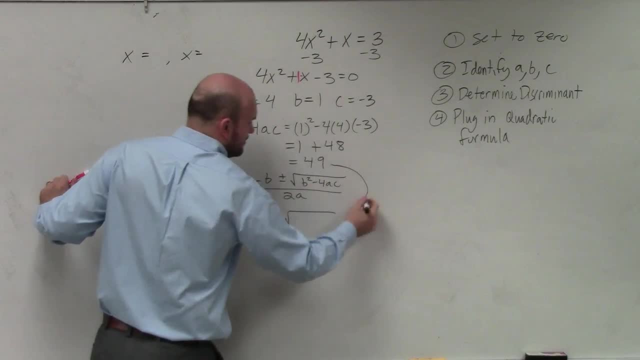 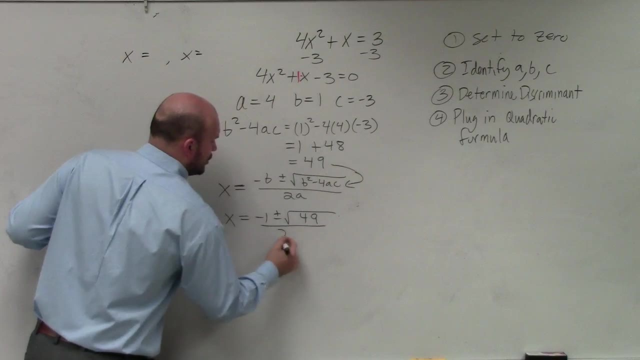 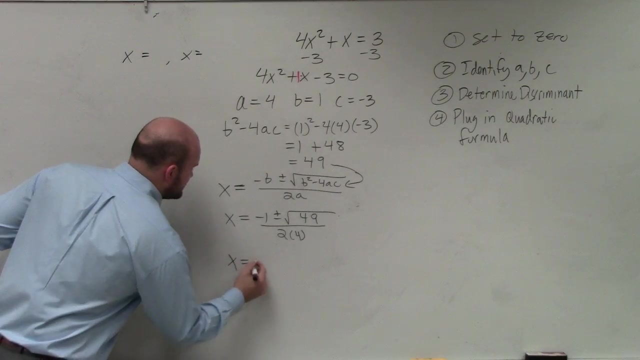 Square root of b, squared minus 4 times a times c. well, that's just going to be the square root of 49, all over 2 times a, which is 4.. So x equals negative 1, plus or minus 7, divided by 8.. 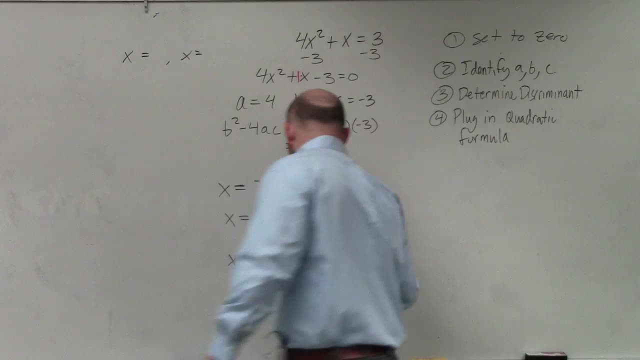 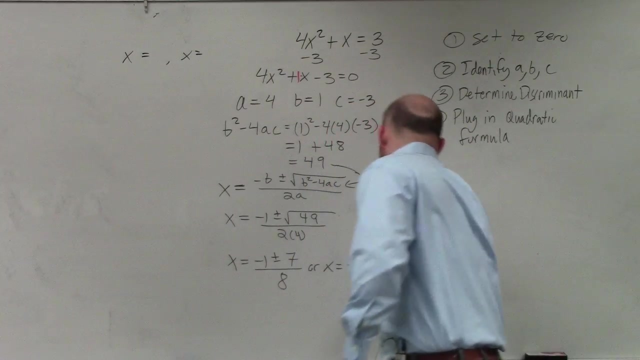 Now we're just going to do this. Now you can separate this into. you could say: x equals negative 1 plus 7 over 8, and negative 1 minus 7 over 8.. So let's go ahead and do that.